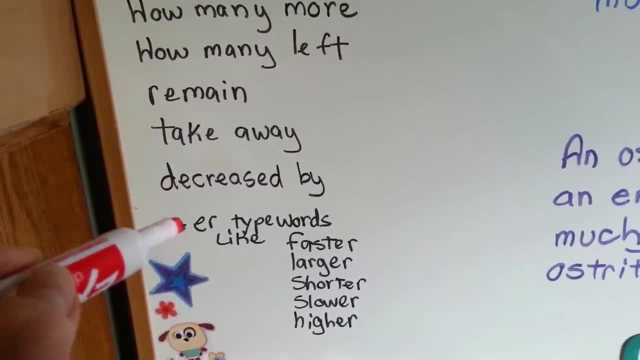 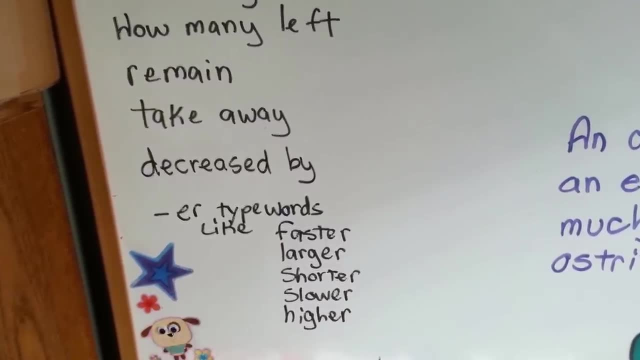 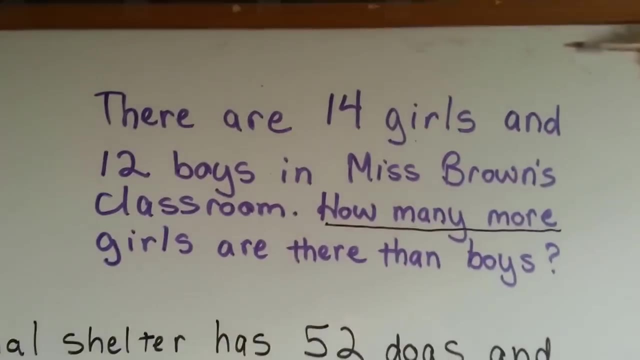 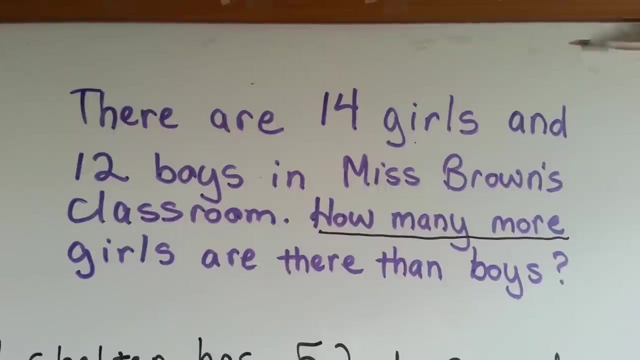 And there are ER words, words that end in ER, like faster, larger, shorter, slower, higher, quicker- Words that end with ER. So let's look at an example. There are 14 girls and 12 boys in Ms Brown's classroom. How many more girls are there than boys? 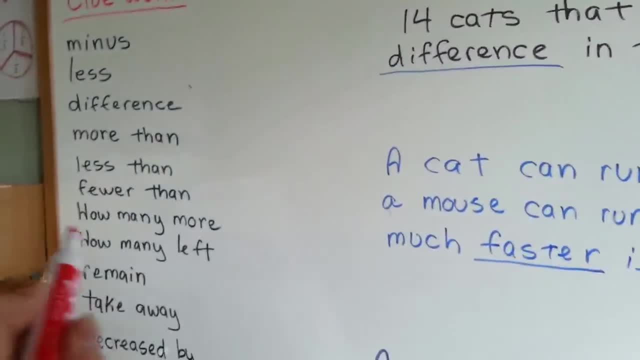 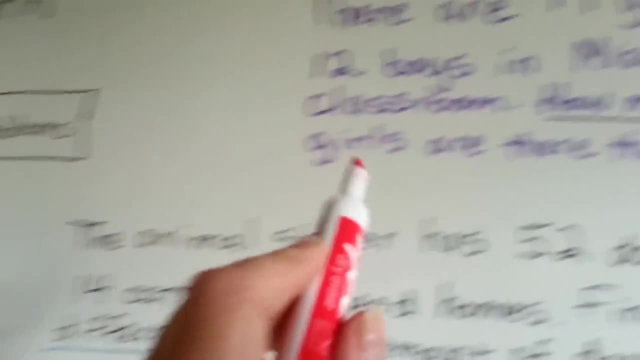 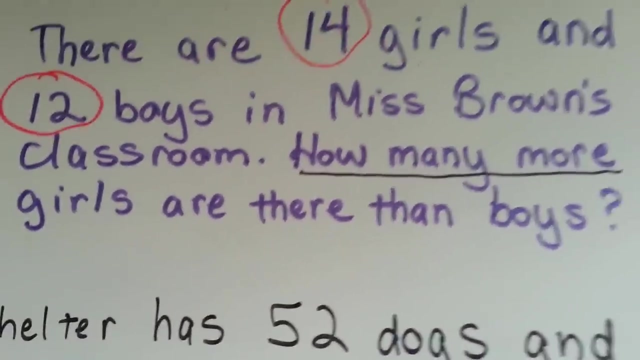 How many more Is a clue word right here. see How many more. So we know it's a subtraction word problem and we need to subtract. So we identify the numbers. We have 14 girls and 12 boys, okay. 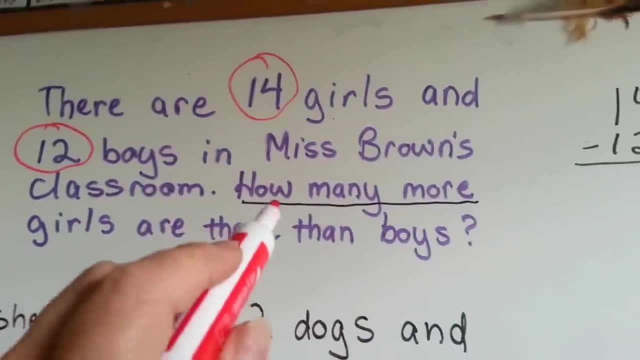 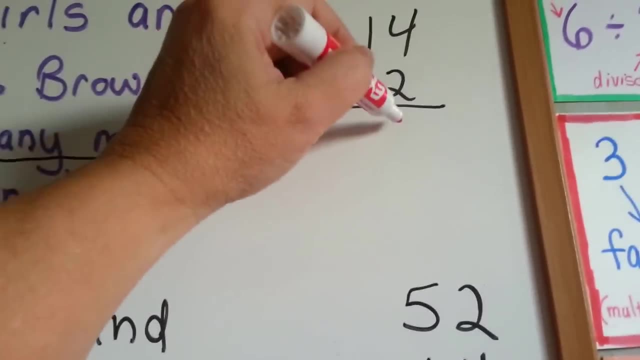 Those are the numbers that we need to subtract, So we're going to have 14 as the minuend and 12 as the subtrahend. 4 take away 2 is 2.. Don't forget, we need to label them. How many more girls? 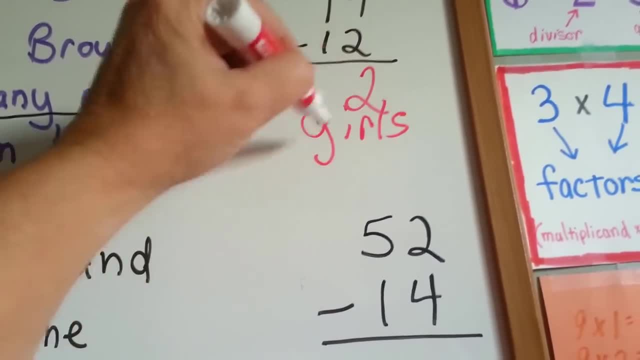 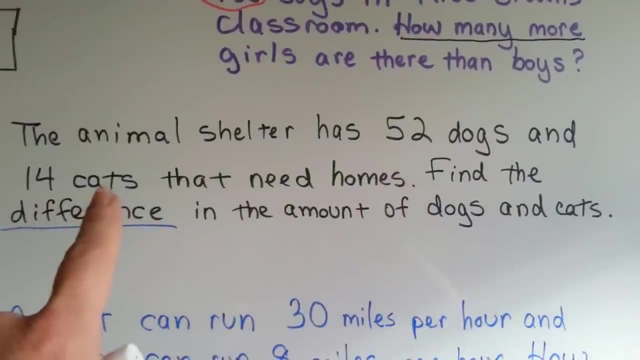 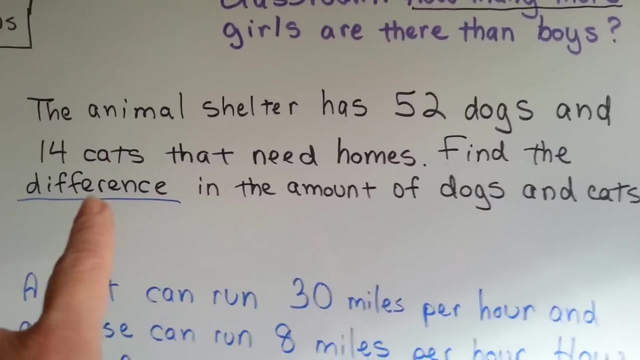 So the answer would be 2 girls. Let's try this one. The animal shelter has 52 dogs and 14 cats that need homes. Find the difference in the amount of dogs and cats. Difference is our clue word. It's right here. 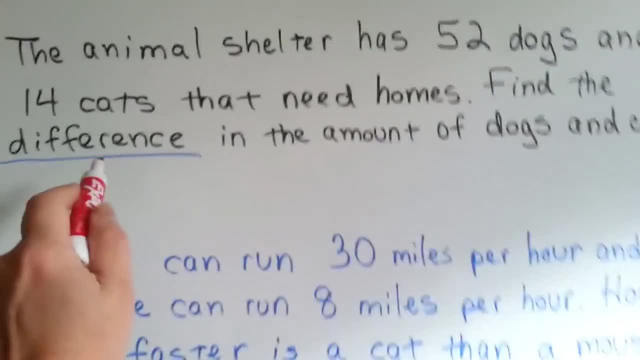 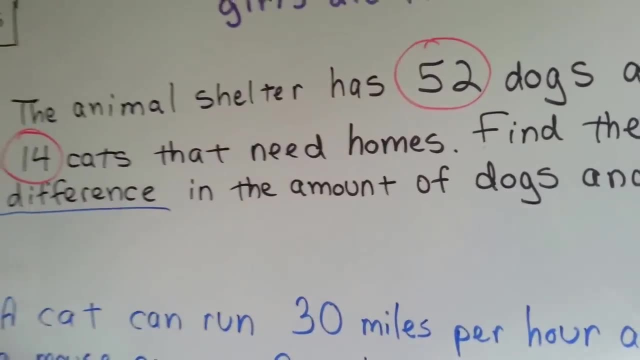 It's a subtraction clue word difference. That's right, It's a subtraction clue word difference. So now what we need to do is identify the numbers 52 and 14.. Those are the numbers we need to subtract and then, don't forget, we need to label. 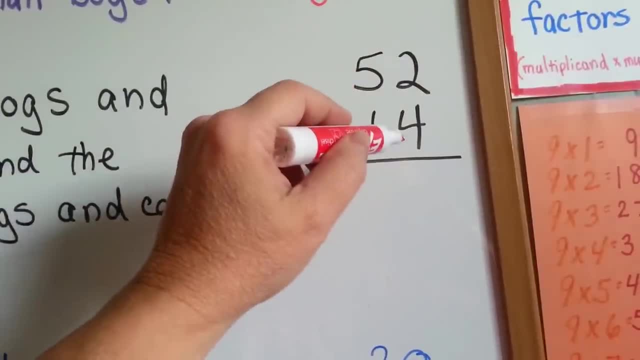 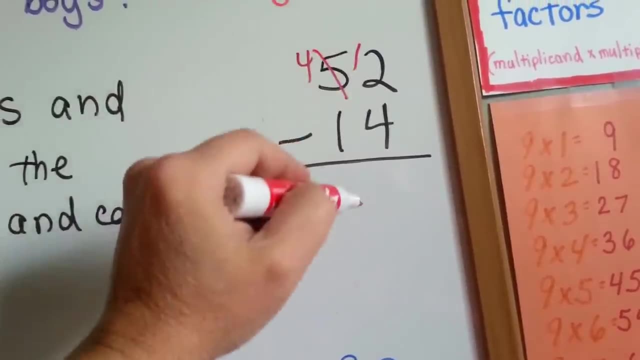 52 minus 14.. Can you have 2 and take 4 away? Nope, So we're going to have to regroup and borrow here: The 5 is going to become a 4, and the 2 is going to become a 12.. 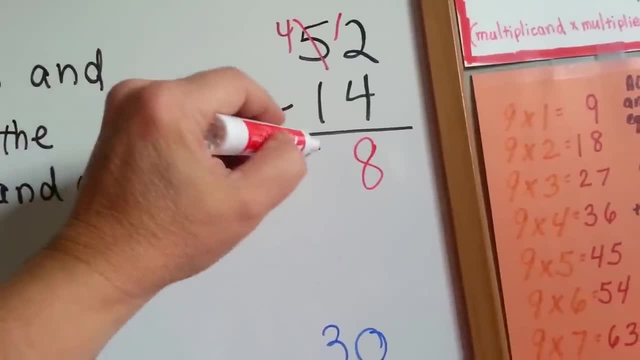 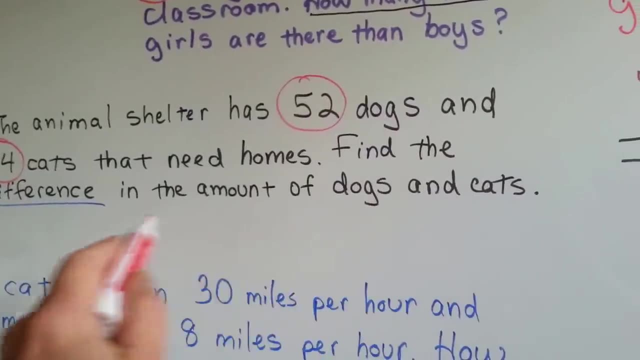 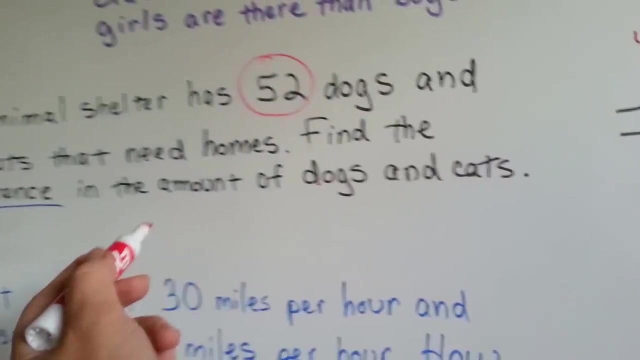 12. take away 4 is 8.. 4. take away 1 is 3.. 30. 38. 38. what Find the difference in the amount of dogs and cats? 38 more dogs, Or you could say 38 less cats. 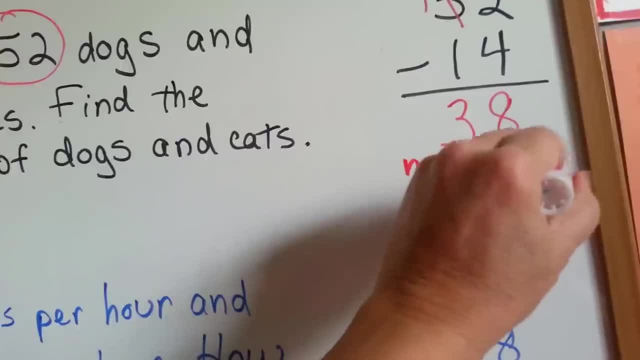 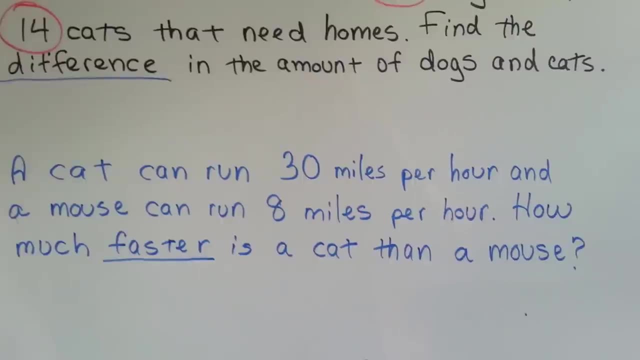 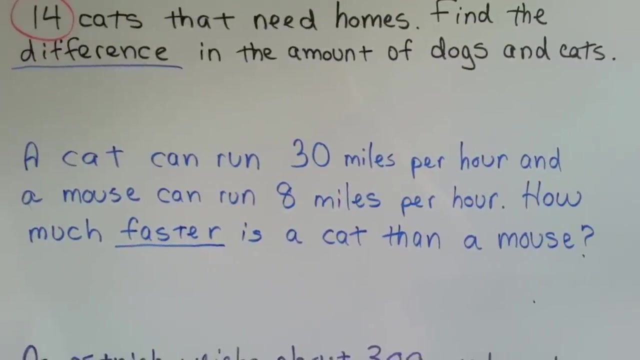 Let's go with more dogs. That's the difference between the amount of dogs and cats. Try this one: A cat can run about 30 miles per hour and a mouse can run about 8 miles per hour. How much faster is a cat than a mouse? 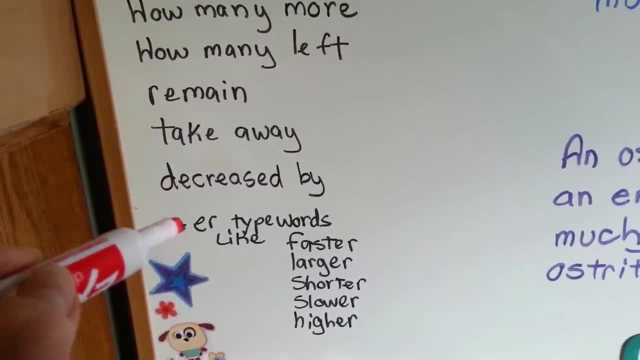 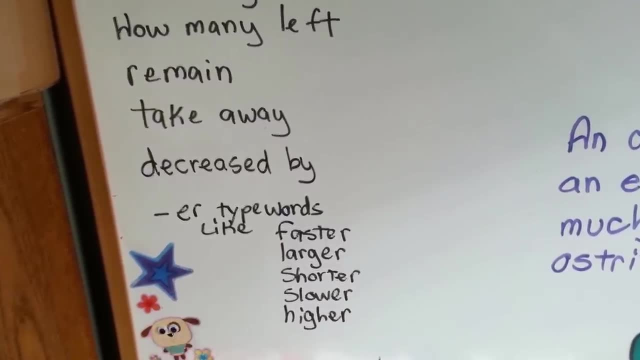 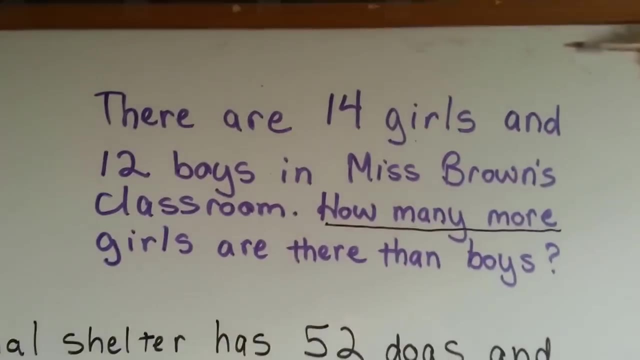 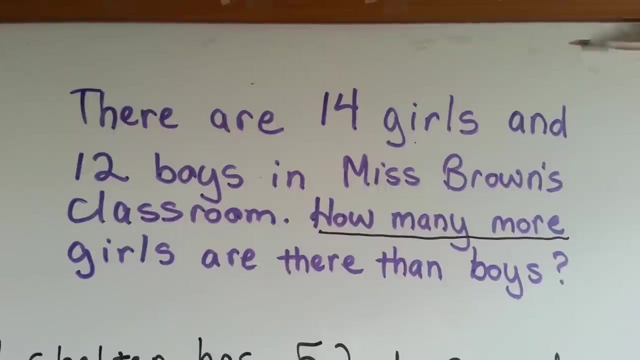 And there are ER words, words that end in ER, like faster, larger, shorter, slower, higher, quicker- Words that end with ER. So let's look at an example. There are 14 girls and 12 boys in Ms Brown's classroom. How many more girls are there than boys? 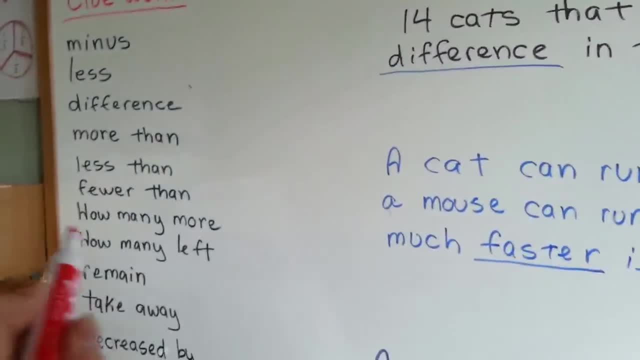 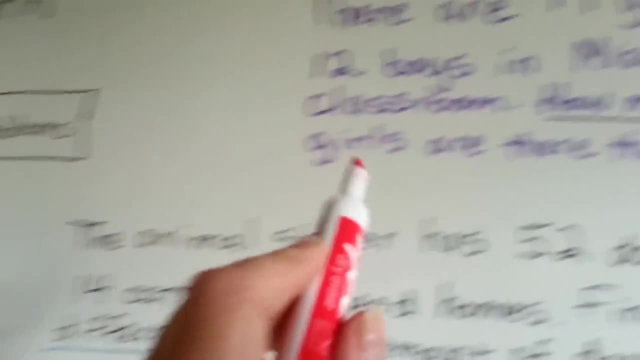 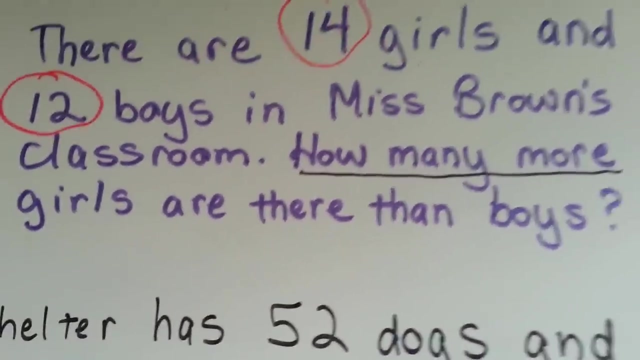 How many more Is a clue word right here. see How many more. So we know it's a subtraction word problem and we need to subtract. So we identify the numbers. We have 14 girls and 12 boys, okay. 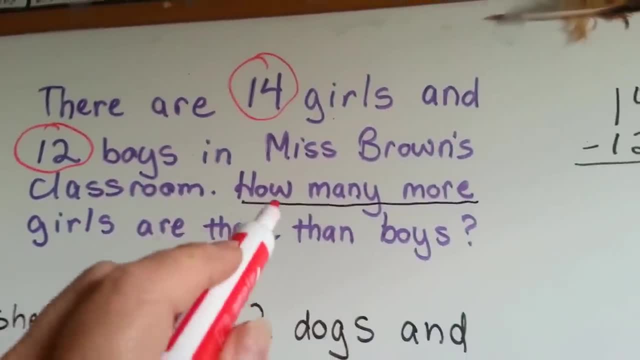 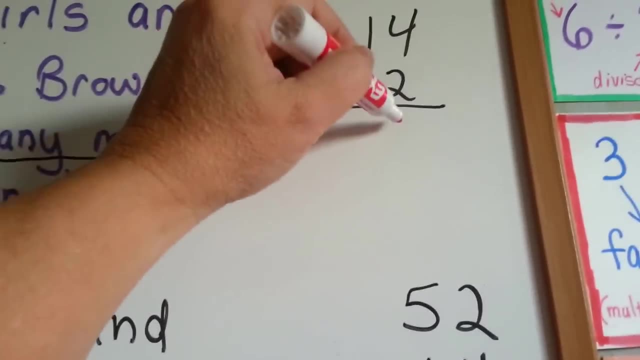 Those are the numbers that we need to subtract, So we're going to have 14 as the minuend and 12 as the subtrahend. 4 take away 2 is 2.. Don't forget, we need to label them. How many more girls? 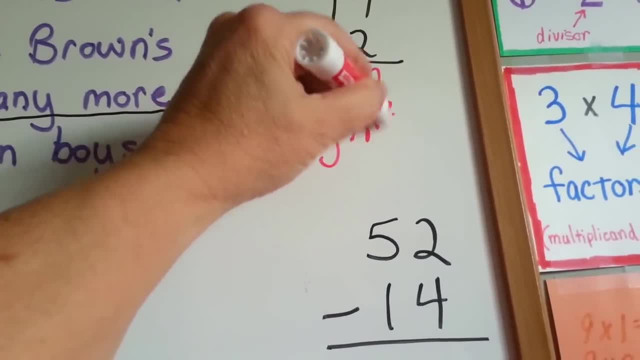 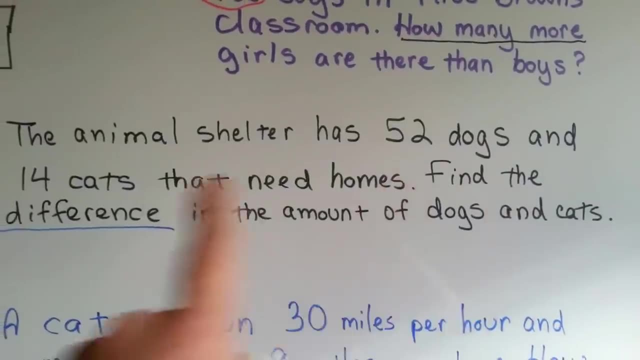 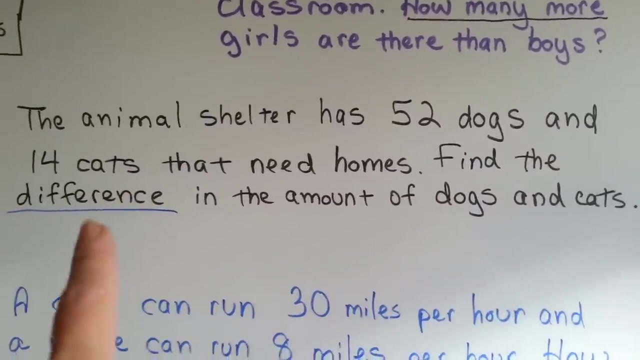 So the answer would be 2 girls. Let's try this one. The animal shelter has 52 dogs and 14 cats that need homes. Find the difference in the amount of dogs and cats. Difference is our clue word. It's right here. 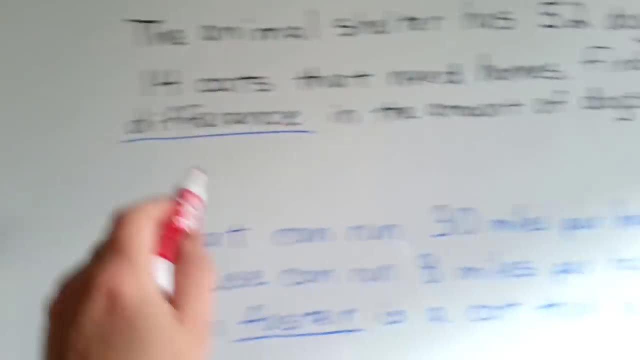 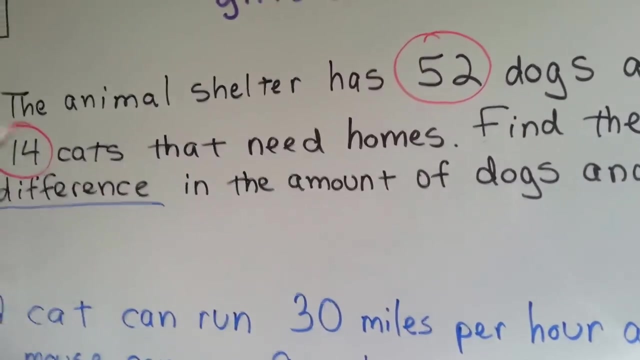 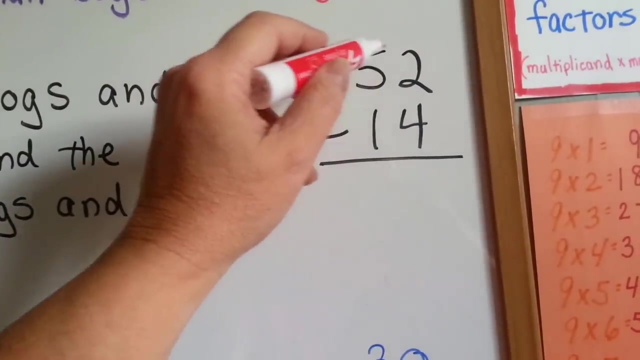 It's a subtraction, clue, word difference. So now what we need to do is identify the numbers 52 and 14.. Those are the numbers we need to subtract and then, don't forget, we need to label 52 minus 14.. Can you have 2 and take 4 away? 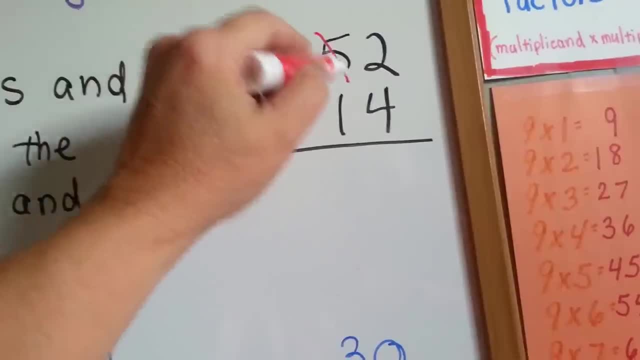 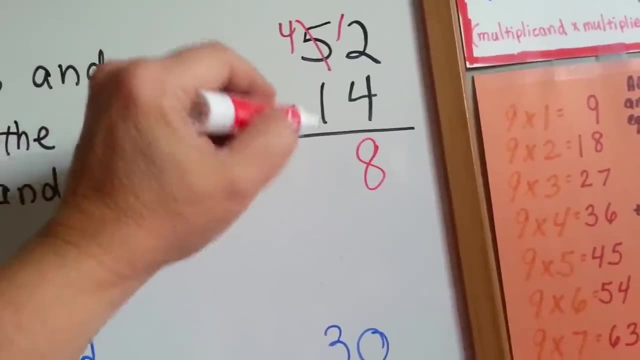 Nope. So we're going to have to regroup and borrow here. The 5 is going to become a 4 and the 2 is going to become a 12.. 12 take away 4 is 8.. 4 take away 1 is 3.. 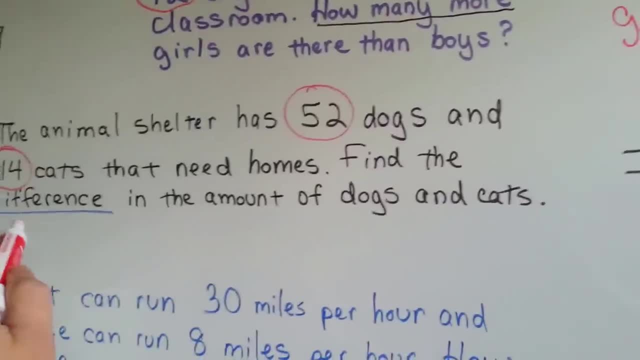 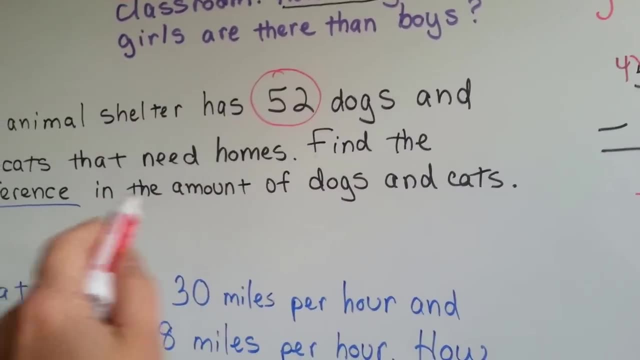 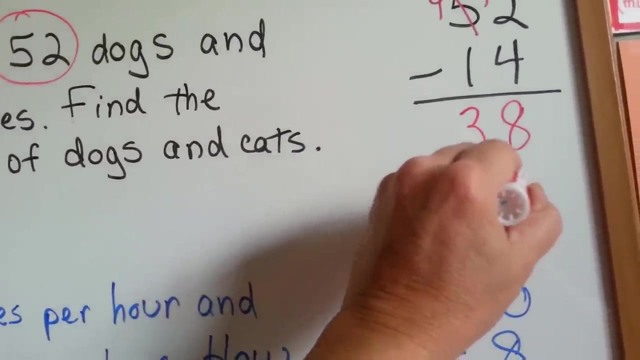 3. take away 2 is 3.. 38. 38. what Find the difference in? the amount of dogs and cats? 38 more dogs, Or you could say 38 less cats. Let's go with more dogs. That's the difference between the amount of dogs and cats. 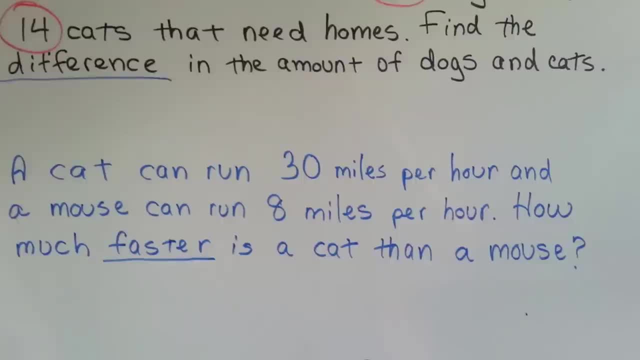 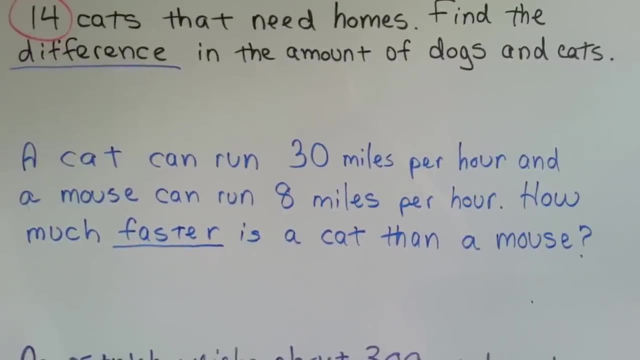 Try this one. A cat can run about 30 miles per hour and a mouse can run about 8 miles per hour. How much faster is a cat than a mouse? Here's our ER word: faster, See, it ends with the ER right here. 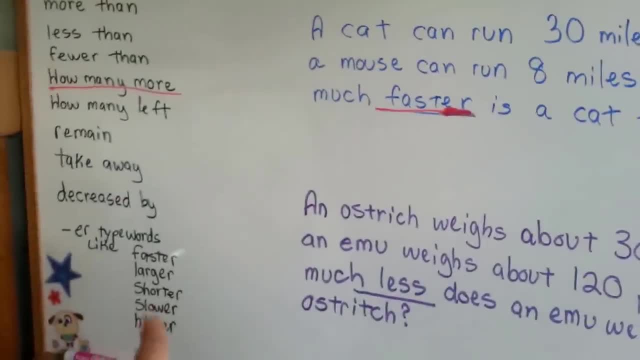 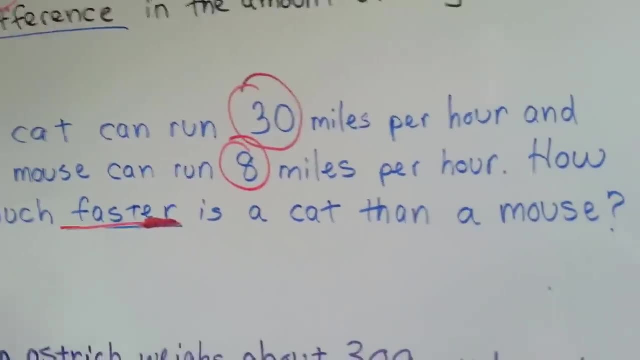 That tells us we need to do subtraction. It's one of the ER words. We're going to identify the numbers 30 and 8 and those are the numbers we're going to subtract. Don't forget we need to label it too. 30 take away 8.. 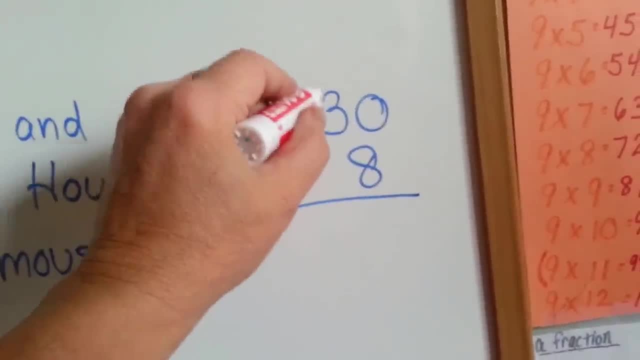 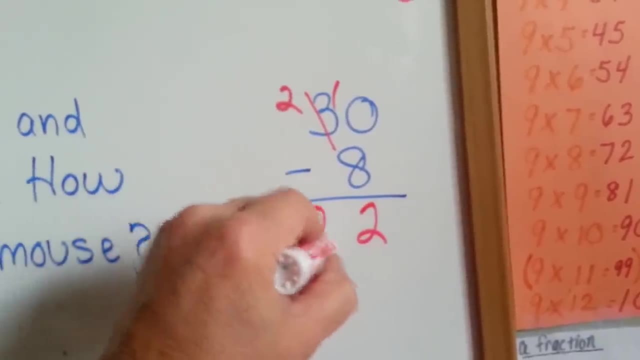 Can you have 0 and take 8 away? Nope, It's going to become a 2 and that's going to become a 10.. 10- take away 8 is 2.. 2- take away nothing is 2. 22.. 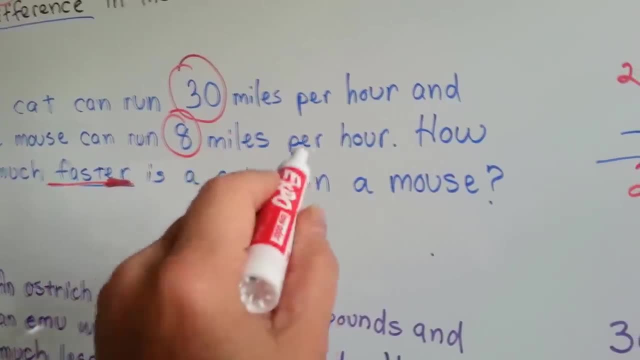 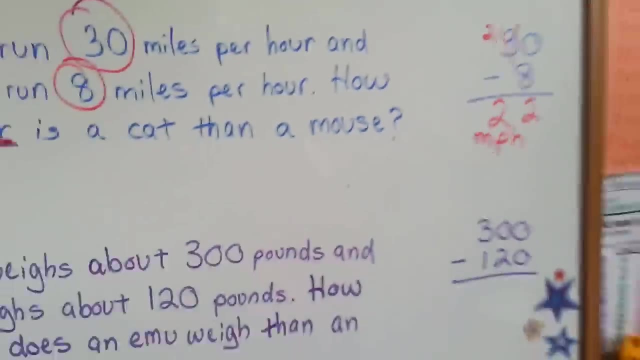 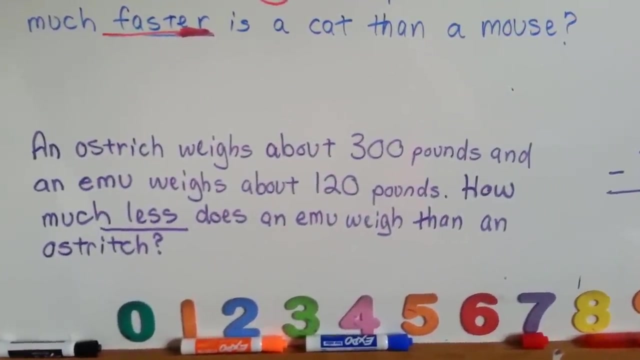 22, what? 22 miles per hour? And you can say MPH for miles per hour. A lot of people write it that way. How about this one? An ostrich weighs about 300 pounds and an emu weighs about 120 pounds. 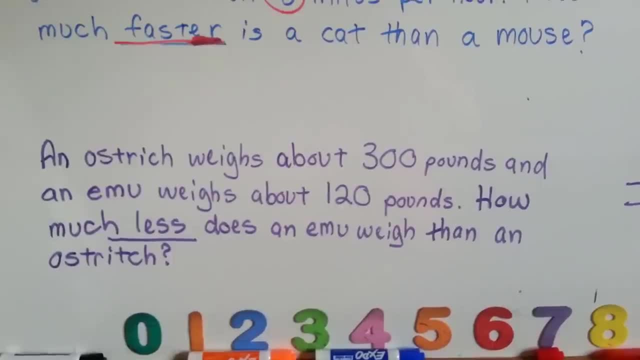 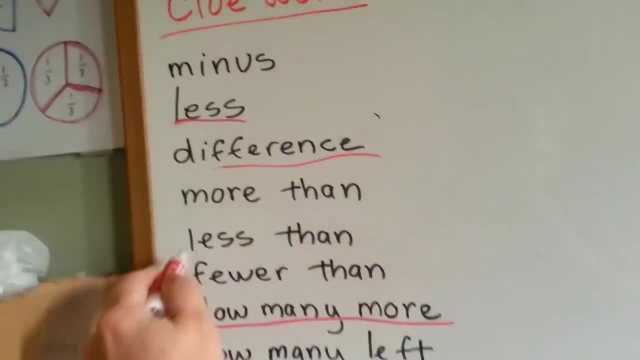 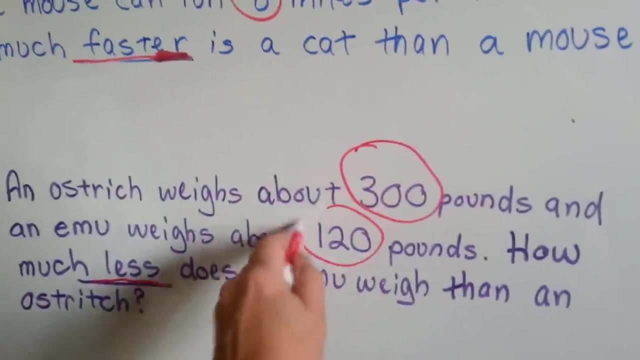 How much less Does an emu weigh than an ostrich? Here's our word: less. That's our clue word. See Less or less than So we're going to identify our numbers 300 and 120.. That's what we need to subtract. 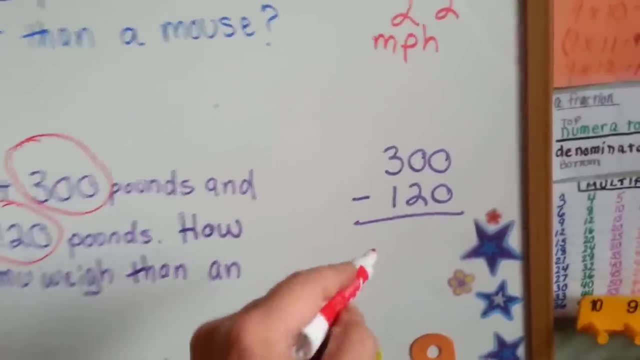 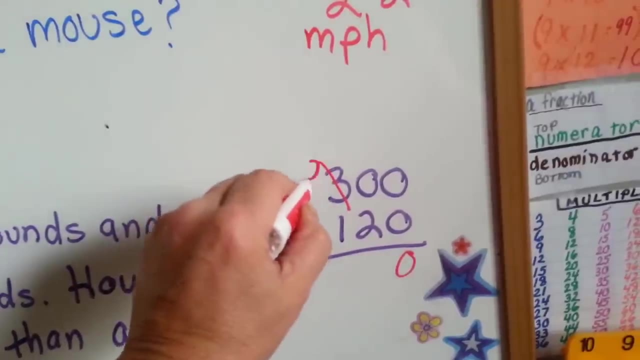 300 minus 120.. 0 take away 0 is 0.. Can you have 0 and take 2 away? Nope. So the 3 is going to become a 2.. That one's going to become a 10.. 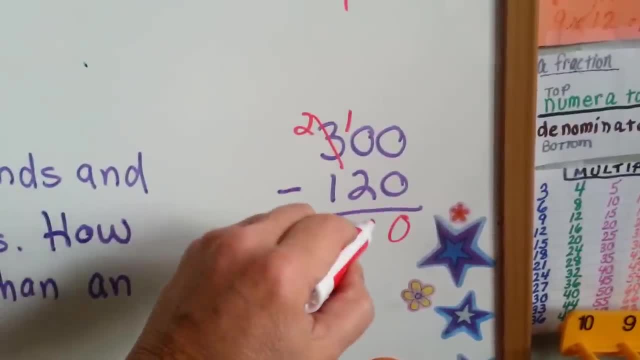 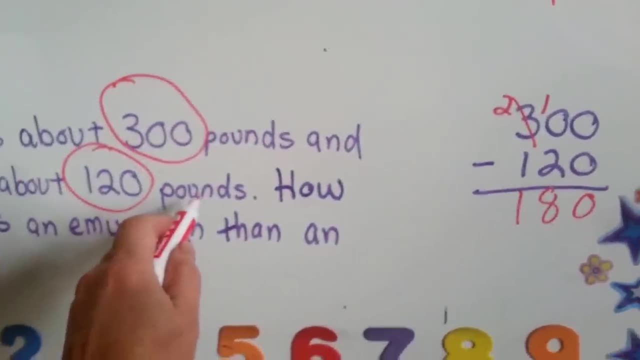 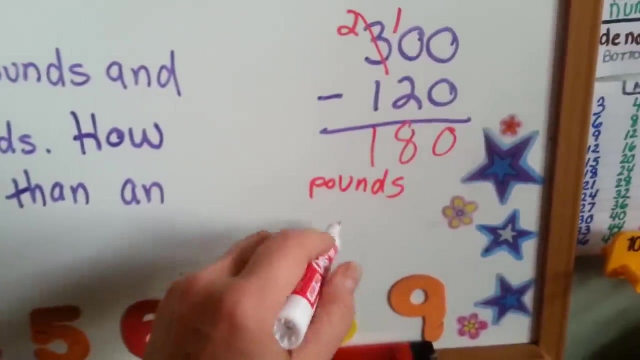 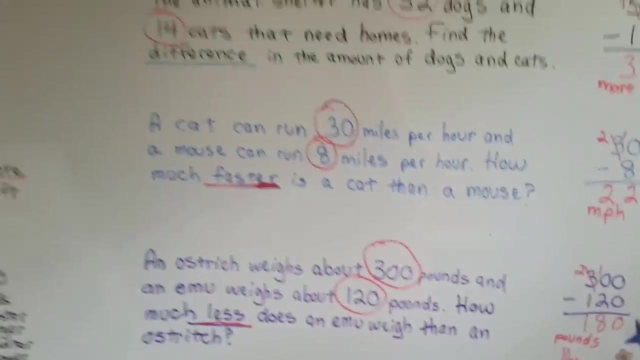 10 take away 2 is 8.. And 2 take away 1 is 1.. 180. what 180 pounds? You can either write pounds or the abbreviation for pounds here in the USA is LBS period, See Subtraction word problems. have clues? 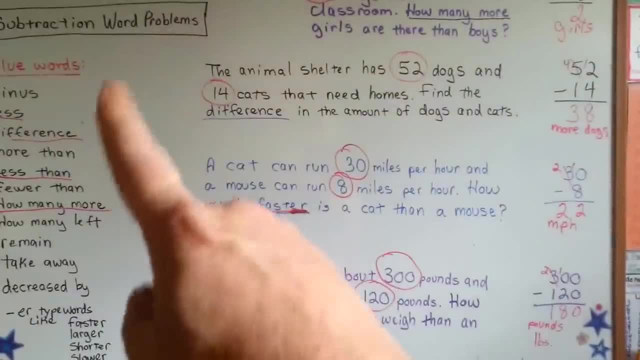 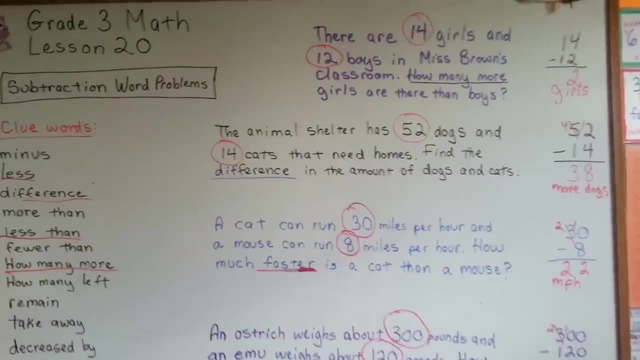 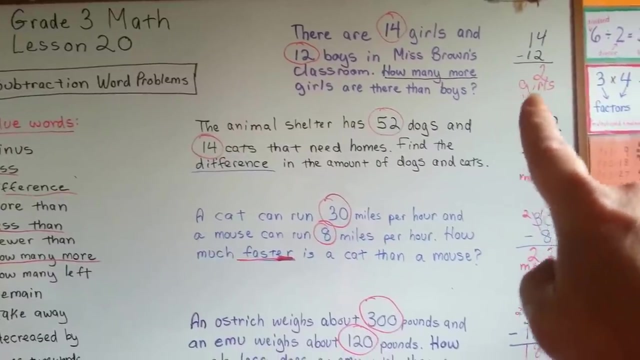 Clue words that tell you to subtract. You might want to make a note of these because these will come up in the word problems. Remember to always identify your numbers, Do your subtraction and label what the answer is. Is the answer more dogs or less cats? 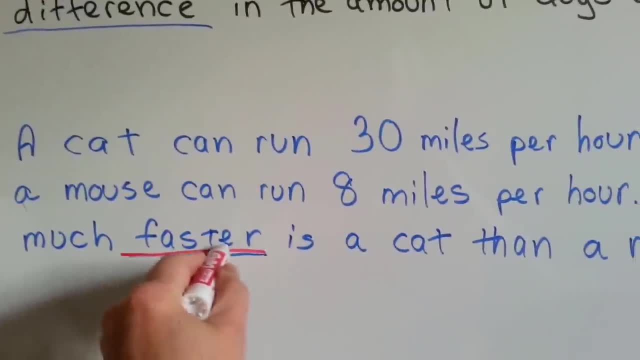 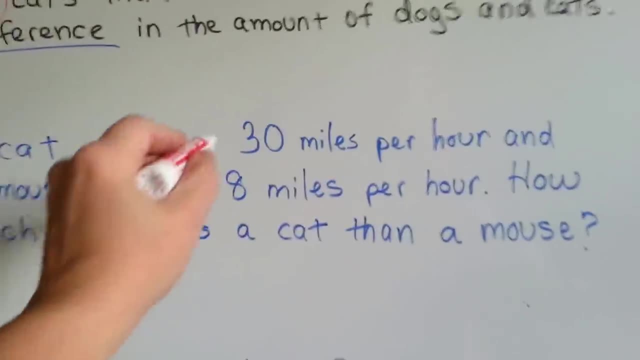 Here's our ER word: faster See. it ends with the ER right here. That tells us we need to do subtraction. It's one of the ER words. We're going to identify the numbers 30 and 8, and those are the numbers we're going to subtract. 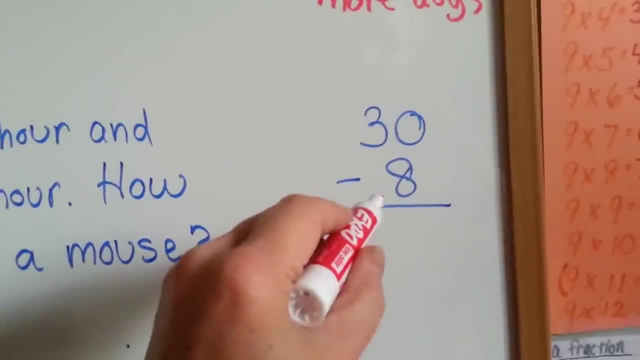 Don't forget, we need to label it too: 30- take away 8.. Can you have 0 and take 8 away? Nope, So that's going to become a 2, and that's going to become a 10.. 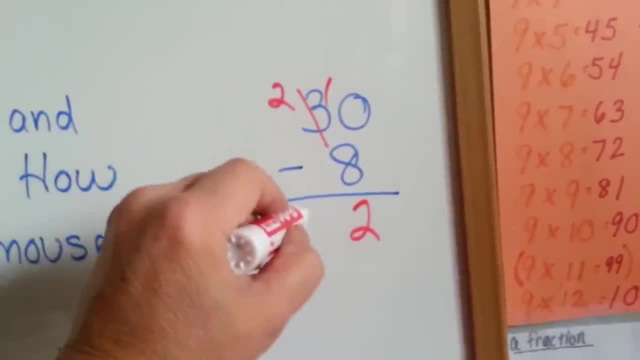 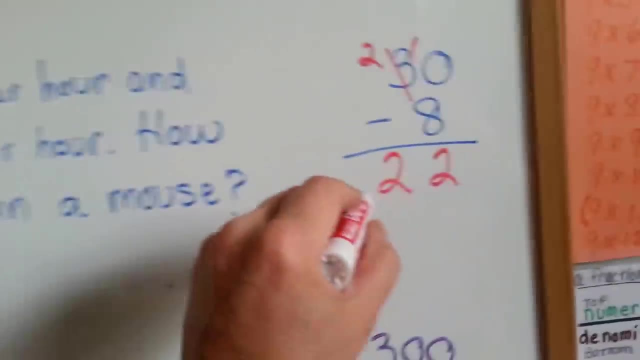 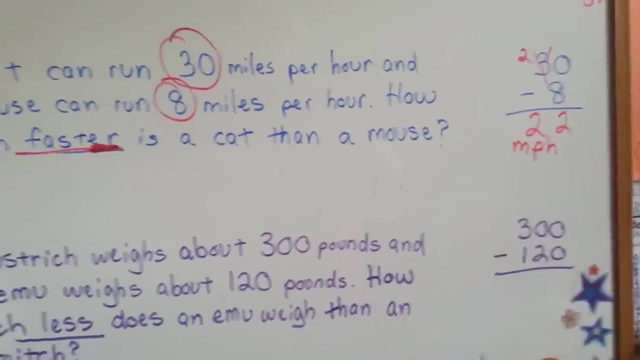 10. take away 8 is 2.. 2. take away nothing is 2. 22.. 22- what? 22 miles per hour And you can say MPH for miles per hour. A lot of people write it that way. 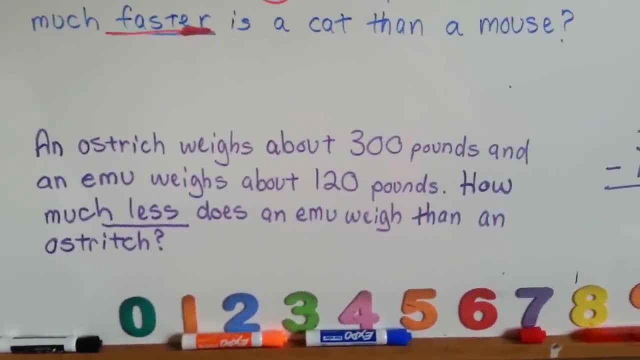 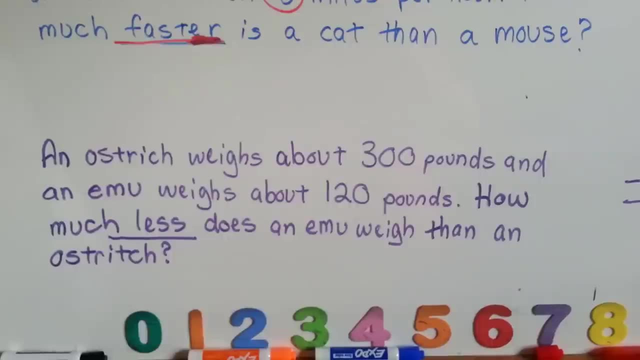 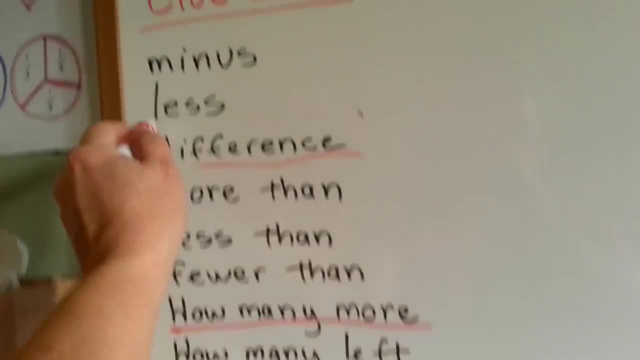 How about this one? An ostrich weighs about 300 pounds and an emu weighs about 120 pounds. How much less does an emu weigh than an ostrich? Here's our word: less, That's our clue word. See Less or less than. 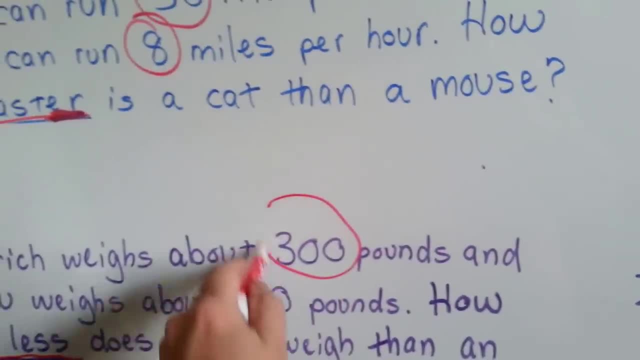 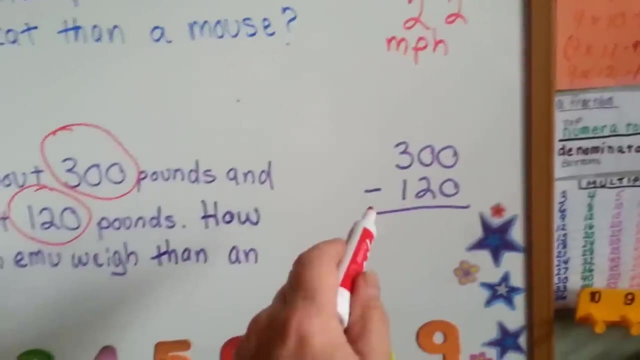 So we're going to identify our numbers: 300 and 120.. That's what we need to subtract 300 minus 120.. 0 take away, 0 is 0.. Can you have 0 and take 2 away? 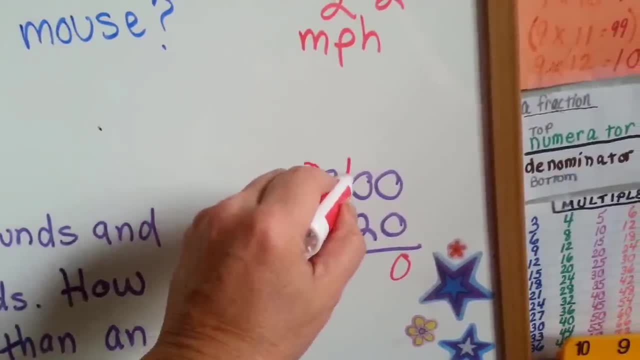 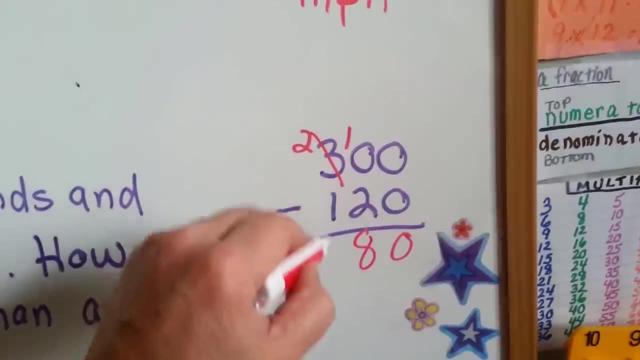 Nope. So the 3 is going to become a 2. That one's going to become a 10.. 10. take away 2 is 8. And 2 take away 1 is 1.. 180. what 180 pounds? 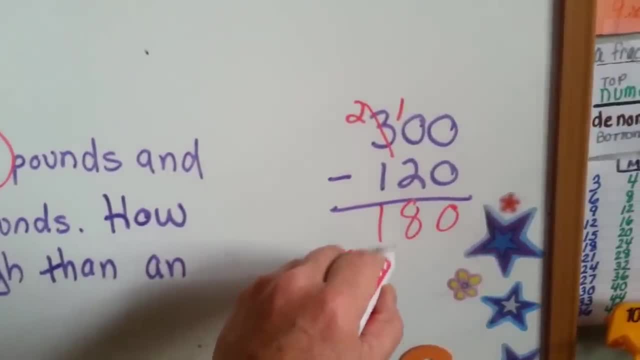 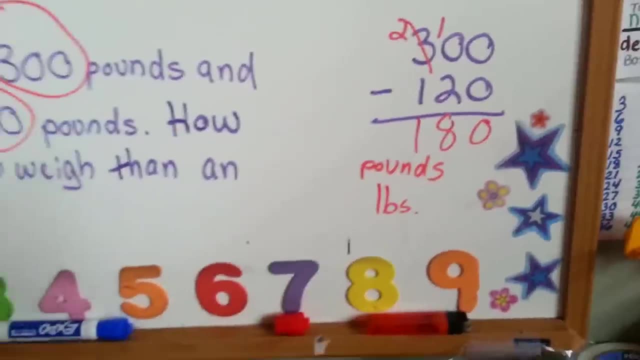 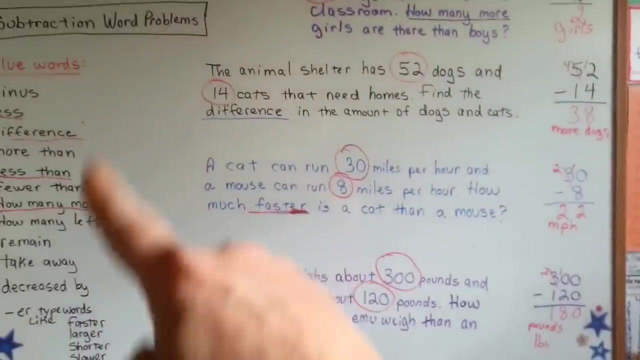 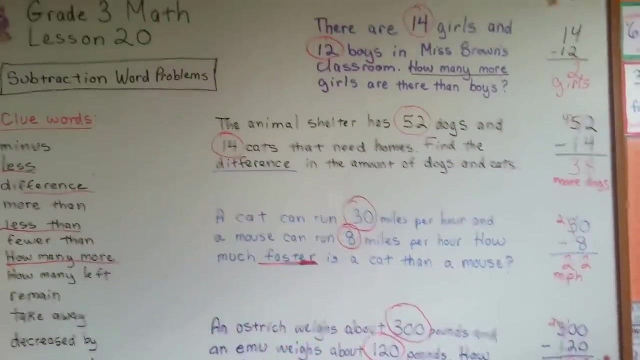 You can either write pounds or the abbreviation for pounds here in the USA is LBS period: See Subtraction. word problems have clues, clue words that tell you to subtract. You might want to make a note of these because these will come up in the word problems. 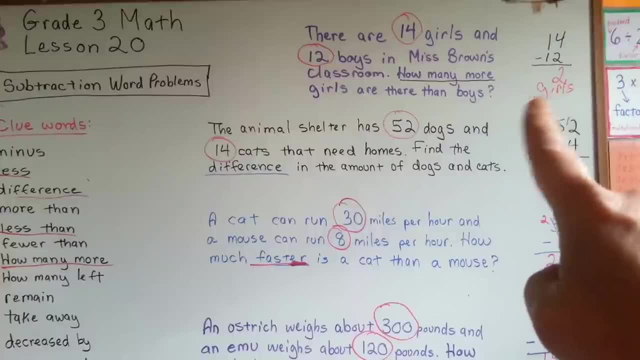 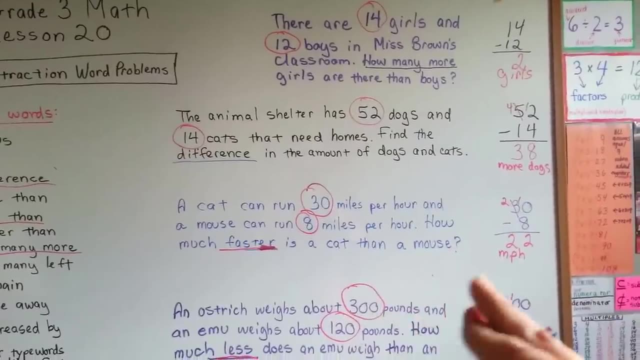 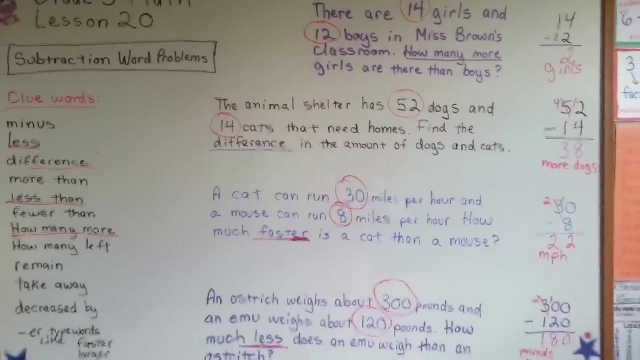 Remember to always identify your numbers, do your subtraction and label what the answer is. Is the answer more dogs or less cats? Is it miles per hour? Is it girls or boys? You have to label your answer in a word. problem, I'll see you next video.